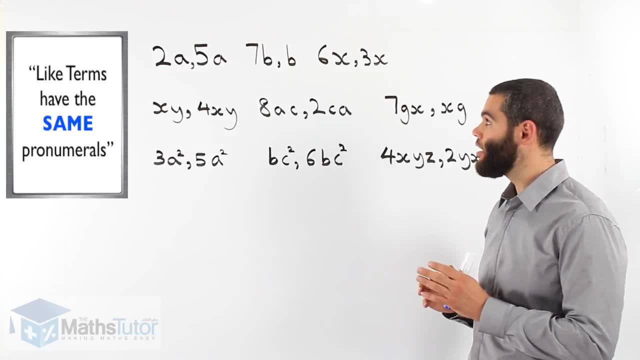 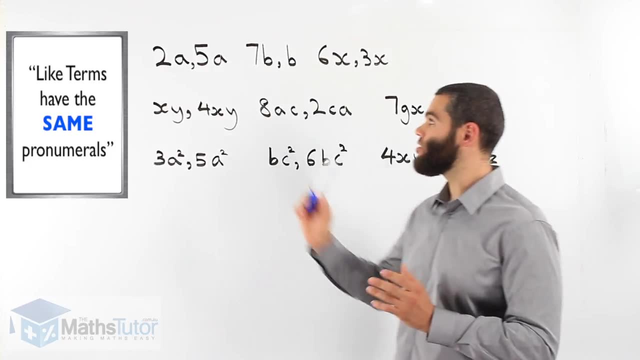 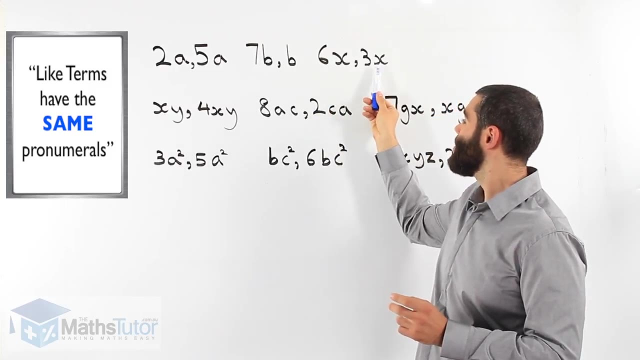 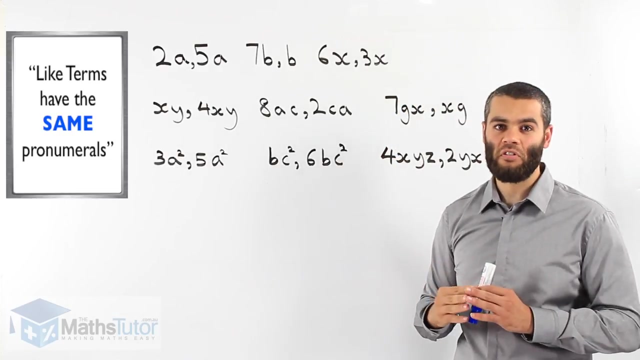 example, and you're going to see what like terms are, Like terms Meaning that the terms have the same pronumerals. Now, what is a term? This is a term: 2a, 5a, 7b, b, 6x, 3x, xy, 4xy, 3a squared, 5a squared. These are all terms To add or subtract. we 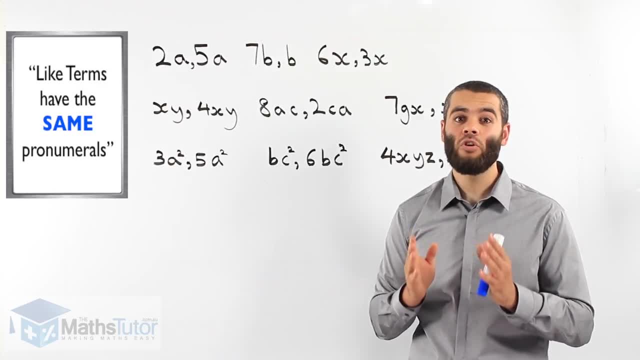 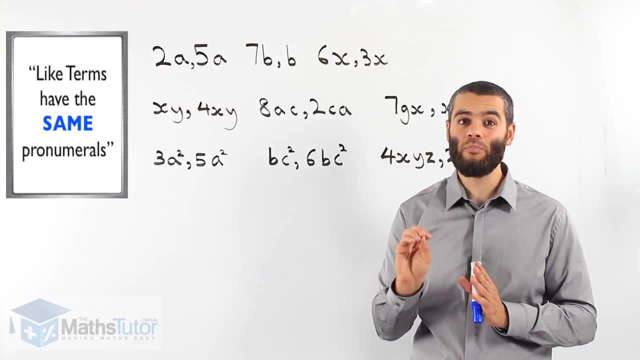 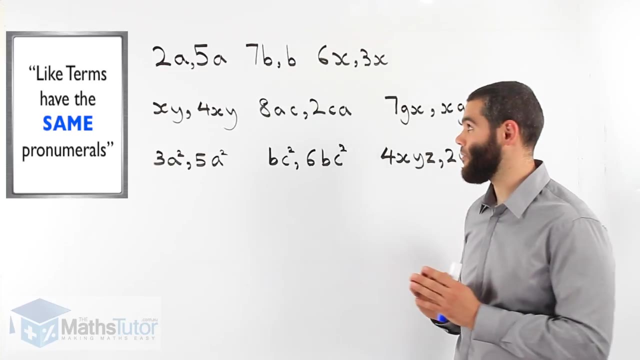 have to make sure we have like terms meaning the same terms, Terms that have the same pronumerals- Very important. If you want to learn anything in algebra that is so important, it's this: You have to only add or subtract like terms. Let's see what like terms are. Now. this is a term 2a and 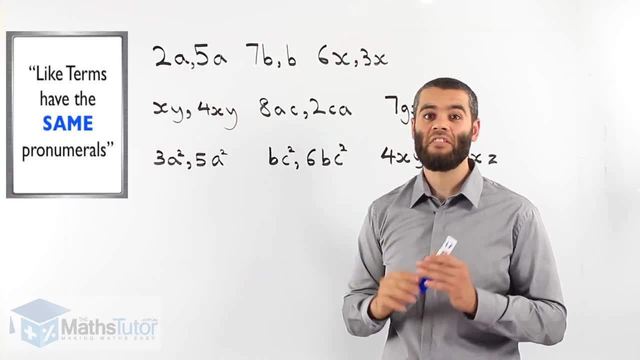 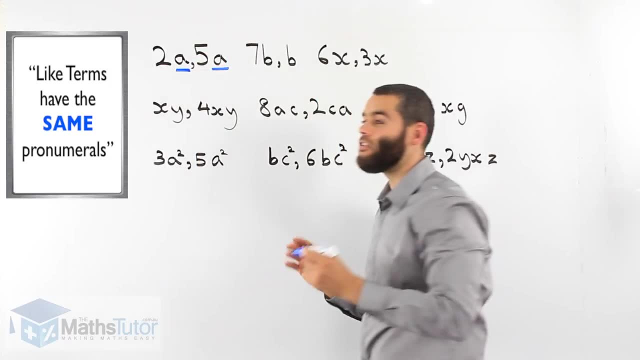 this is 5a. Are they like terms? The answer is yes. Why? Because they have the same pronumerals, A and a, So 2a and 5a. I like to tell students that think of it this way: Two apples and. 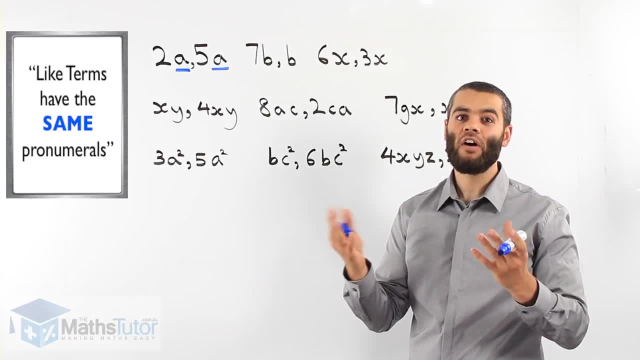 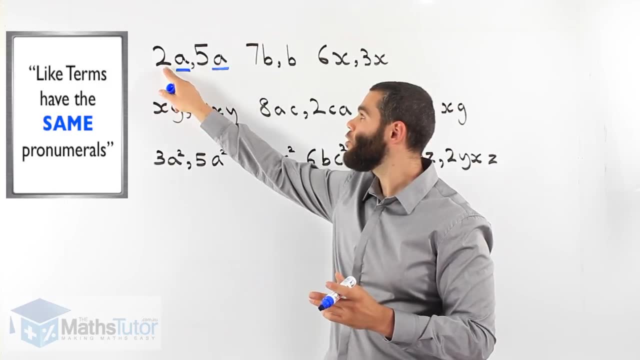 five apples. you can add them up: Two apples, five apples, A for apples, So a pronumeral and a pronumeral. they are the same here and here. Therefore, 2a and 5a are like terms. 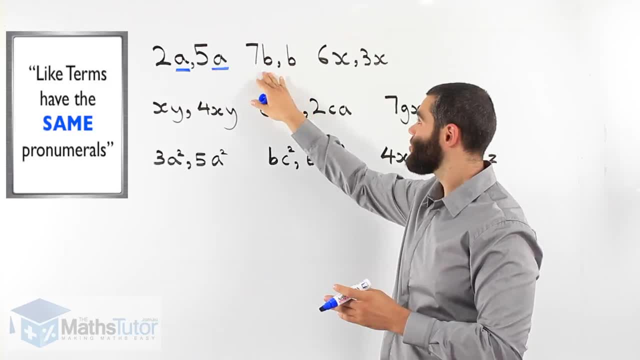 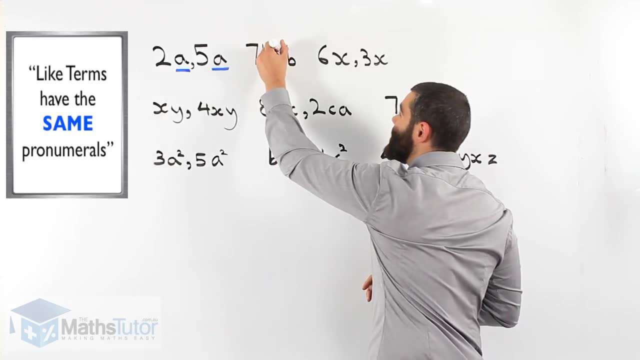 So you can add them up. Are these like terms? We have 7b and we have b. Now b really means that there's a 1 here, One b. So when you see a b, It's not just a b. 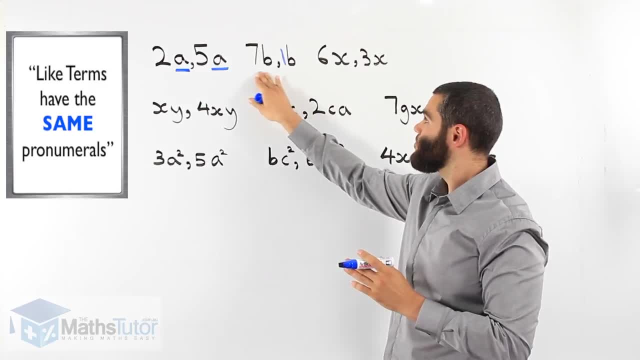 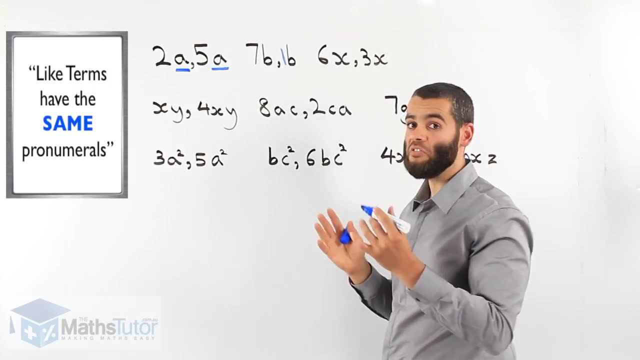 it's actually 1b. Are these like terms? Do they have the same pronumeral? That's the question you ask. Do they have the same pronumeral or pronumerals In this case? here, yes, they have a b. 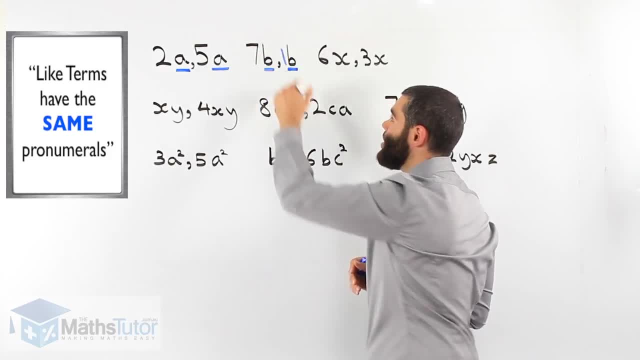 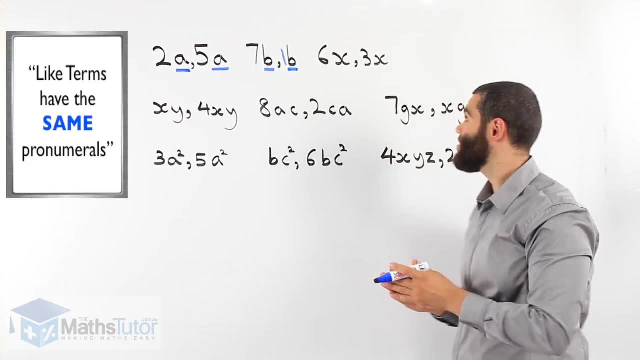 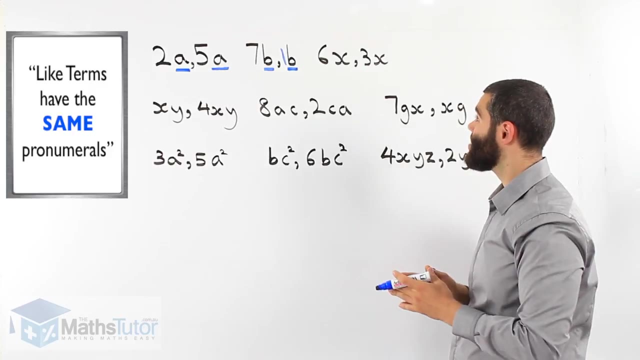 and a b. Therefore, 7b and b are like terms. Now you answer this one: 6x and 3x Are they like terms? What do we ask? Do they have the same pronumeral? The same pronumeral? we have an x. 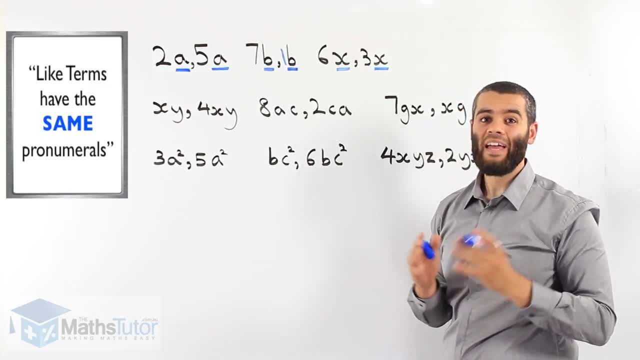 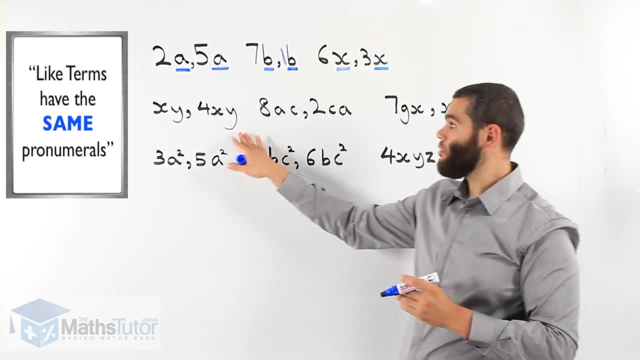 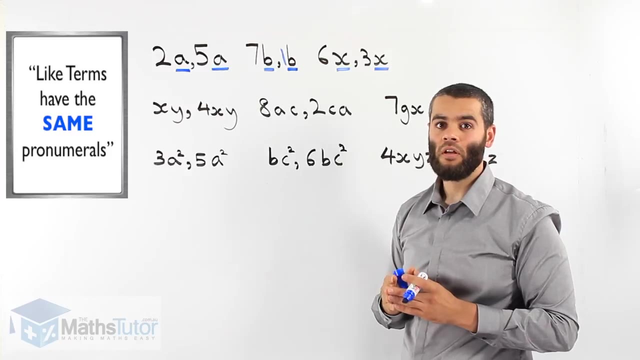 here and an x here. Yes, 6x and 3x are like terms, meaning they can be added and subtracted. Looking here we have: xy is one term and 4xy is another term. Are they like terms? We ask? 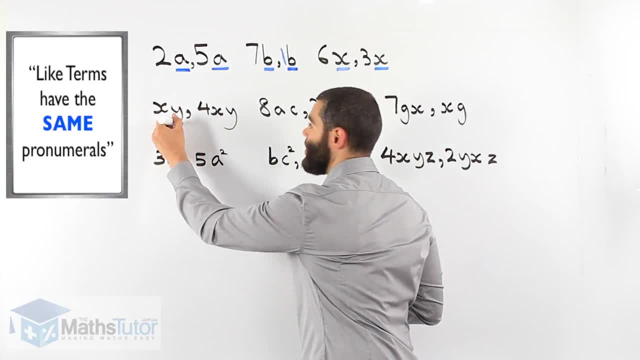 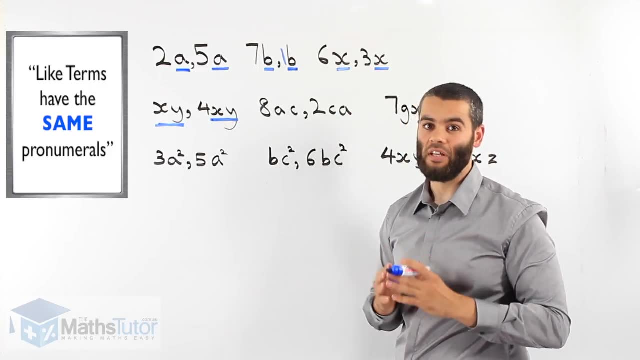 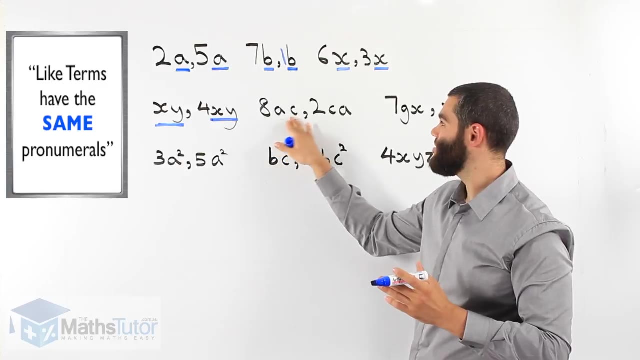 well, do they have the same pronumerals? We have an xy here and an xy here. Yes, they are like terms, so we can add them up if we need to: 8ac- 2ca. We have a term here, 8ac, another term, 2ca. Are they like terms? Let's see, Do they have? 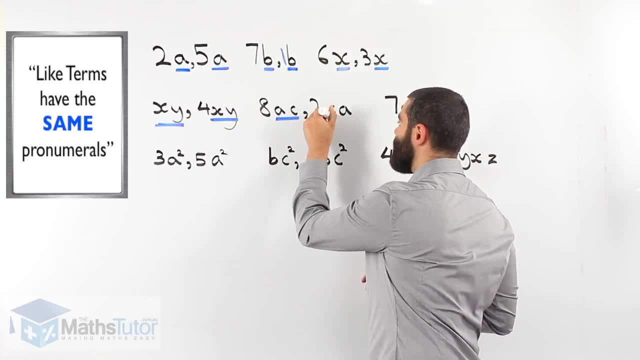 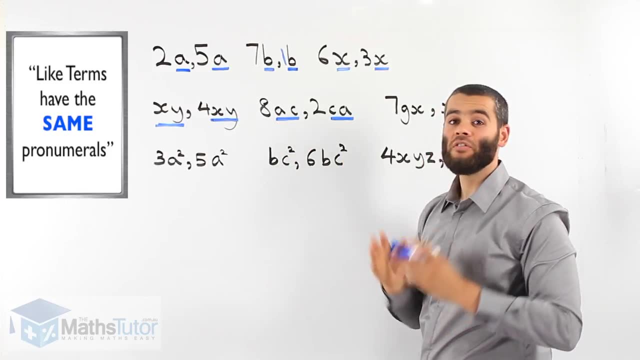 the same pronumerals. We have ac here and we have ca here. They have the same pronumerals. However, they have been swapped. Do they have the same pronumerals? Yes, they have the same pronumerals. They have been swapped. ac- ca Doesn't matter as long as they have the same pronumerals. The order. 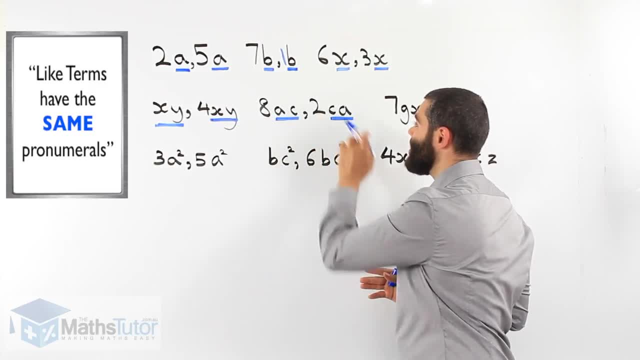 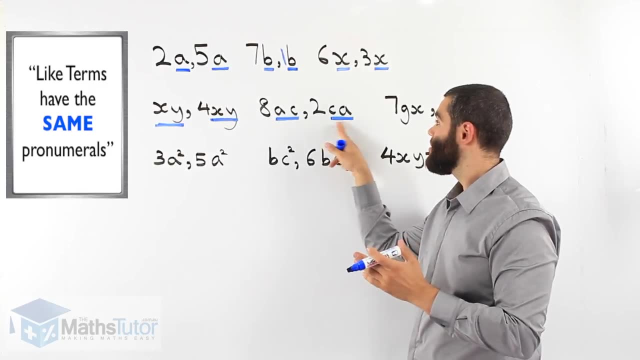 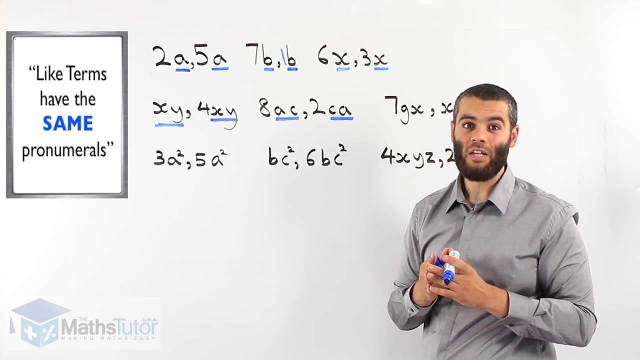 does not matter at all- ac, ca And we learnt before that ac means a times c and c times a ca. So we're multiplying 4 times 3 and 3 times 4. It's the same answer anyway. You get 12.. 4 times. 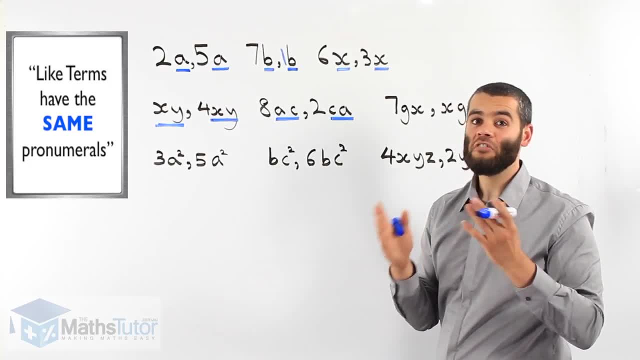 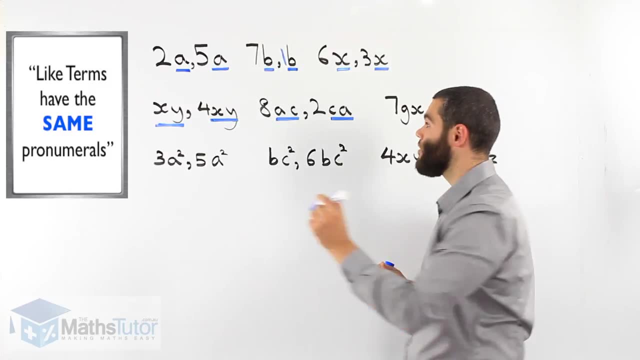 3 is 12, and 3 times 4 is 12.. So the order is the same, Does not matter. So ac a times c, ca, c times a, it's the same. Therefore, as long as the 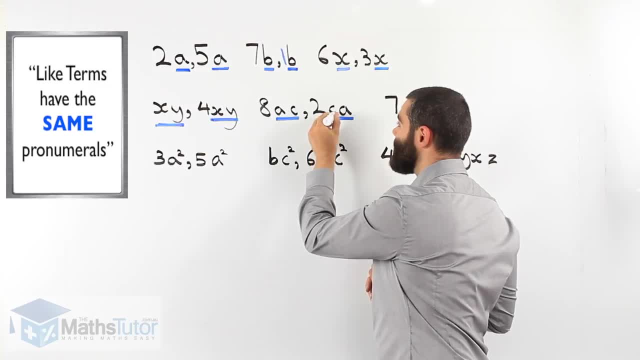 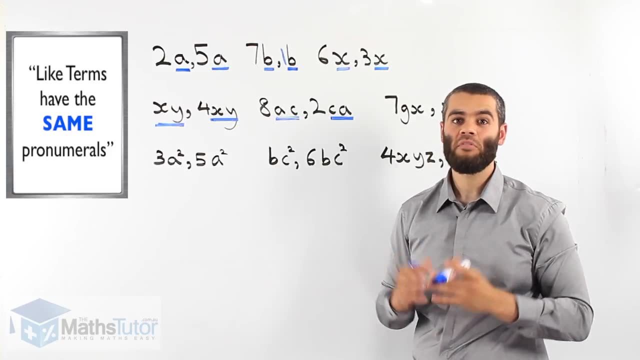 pronumerals are the same. there's an a here and an a there, a c and a c. Yes, they are like terms. 8ac and 2ac or 2ca are like terms. They can be added or subtracted if we need to. 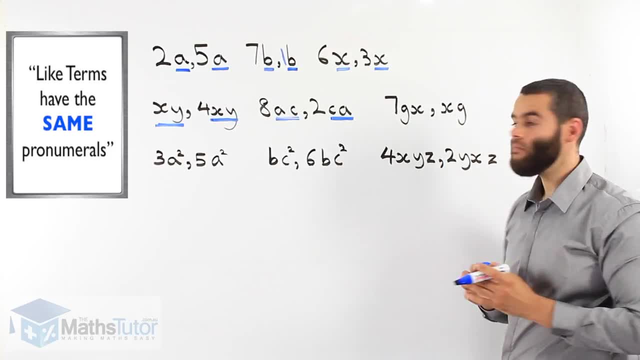 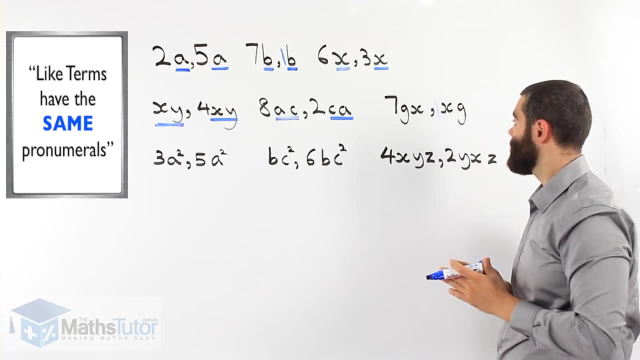 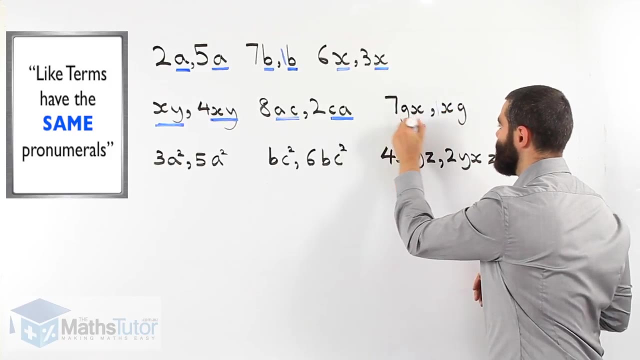 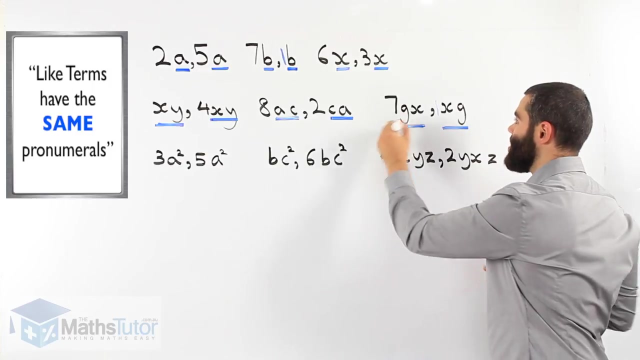 Here, 7gx is one term, There it is, And xg or 1xg is another term. Are they like terms? Well, do they have the same pronumerals: gx, xg? Yes, they do, The order does not matter: x, gx here and xg there. Yes, 7gx and 1xg are like terms. 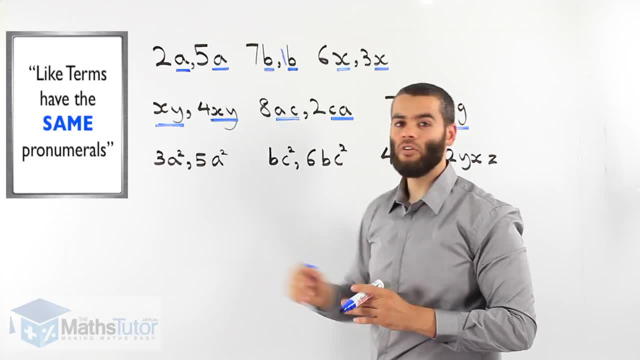 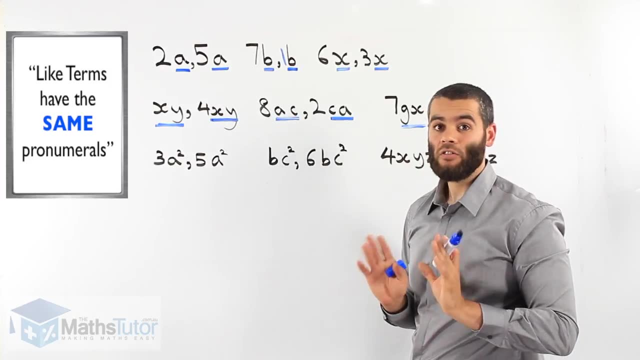 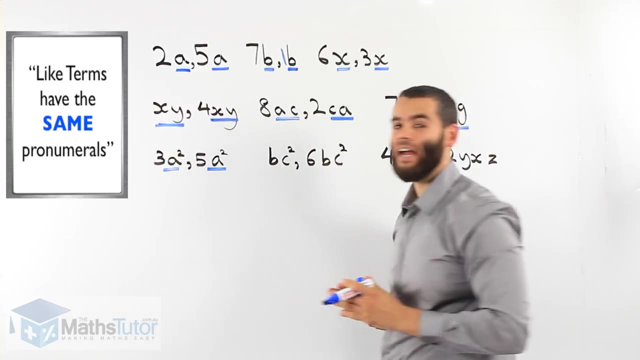 Coming. here we have: 3a squared is a term, 5a squared Is another term. Are they like terms though? Well, do they have the same pronumerals, a squared and a squared? Yes, they have the same pronumerals. Therefore, 3a squared and 5a squared are also. 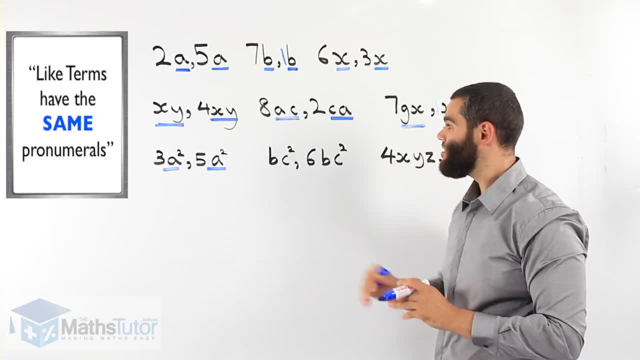 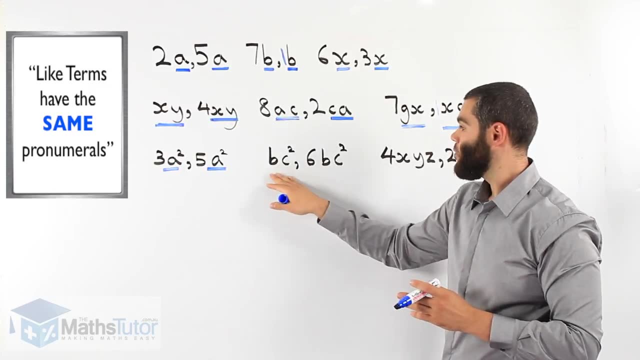 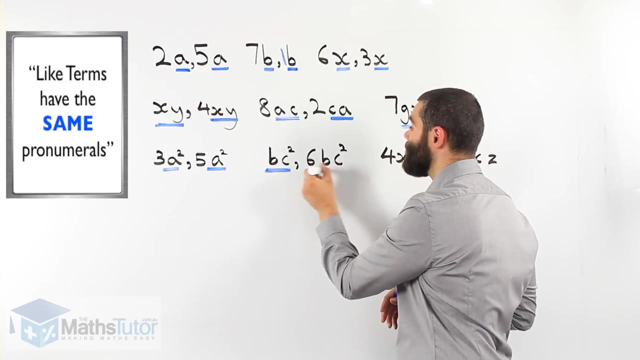 like terms. bc squared is another example, and we have 6bc squared These here. we ask: are they like terms? Well, we have bc squared here, We have 6bc squared here. So we have a bc squared and a bc squared. 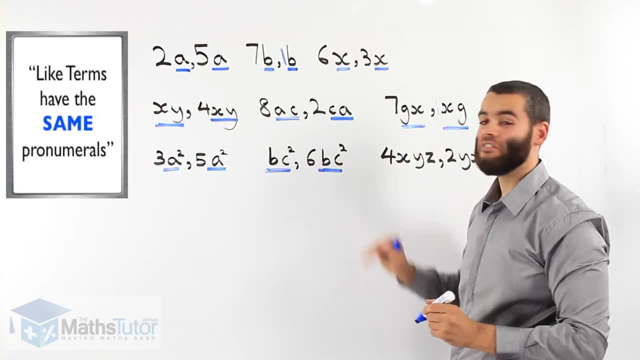 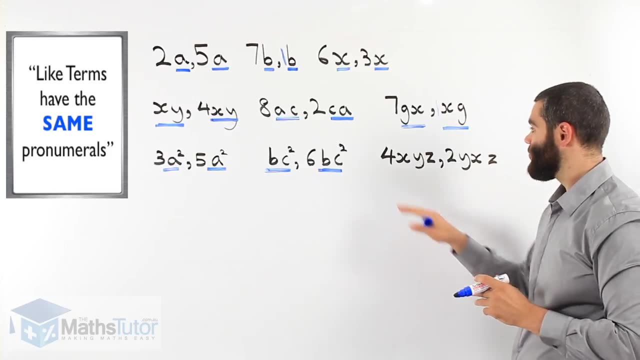 Yes, bc squared and 6bc squared are like terms. They can be added or subtracted. Last example: 4xyz is a term and 2yxz is another term. We ask: Are they like terms? Well, do they have the same pronumerals? They can be added or subtracted if we need to. 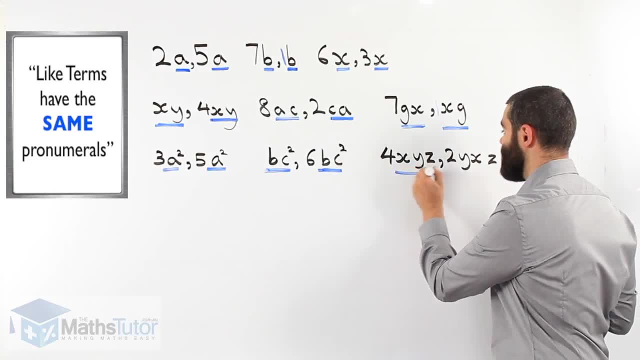 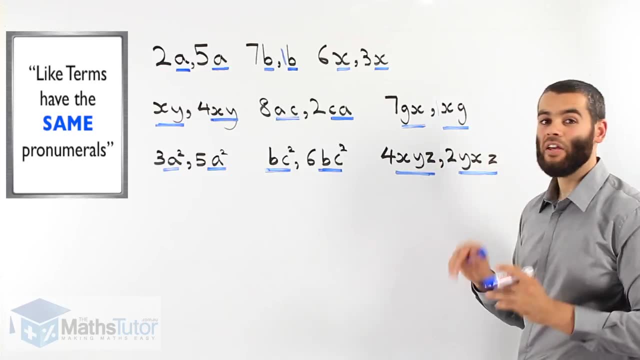 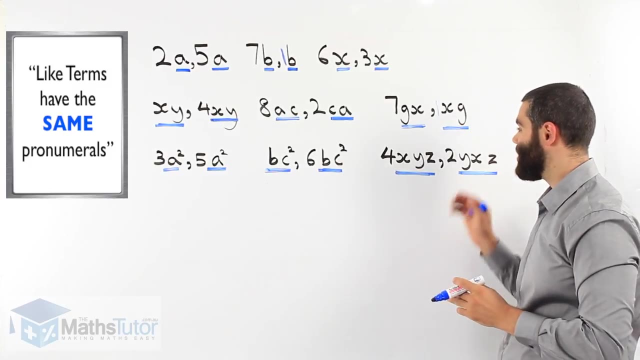 Are they like terms? Well, x 찾. here they're the pronumerals ychz. we have an x, yes, we have a y. yes, we have a z, yes. Therefore, 4xyz and 2yxz are like terms. That means we can add them or subtract them if 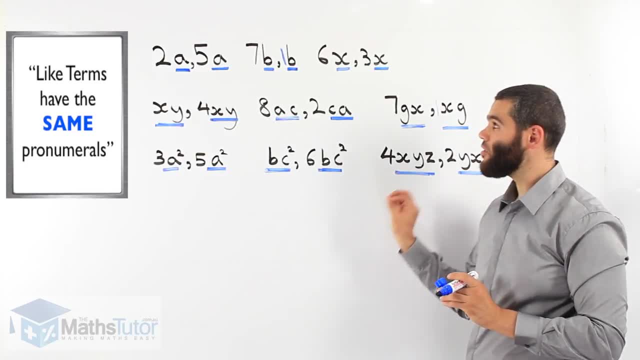 we need to A very important rule: like terms- we now can see what like terms are. And I want to, I want to test you, I'm going to put some here and see whether it's more like or less like. Very important rule: Like terms- we now can see what like terms are. And I want a little. I 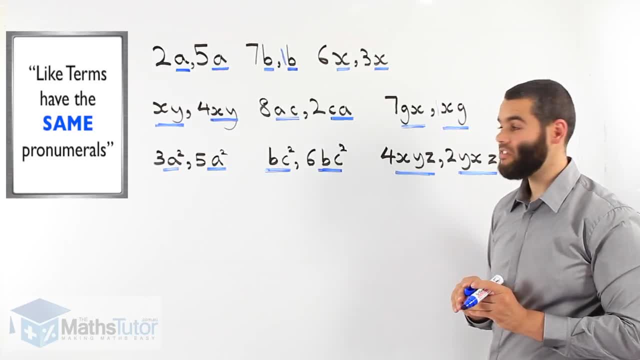 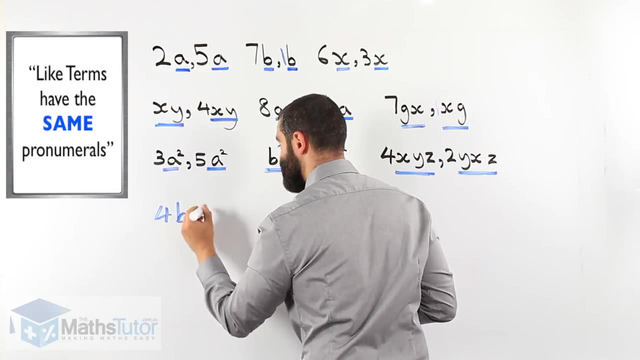 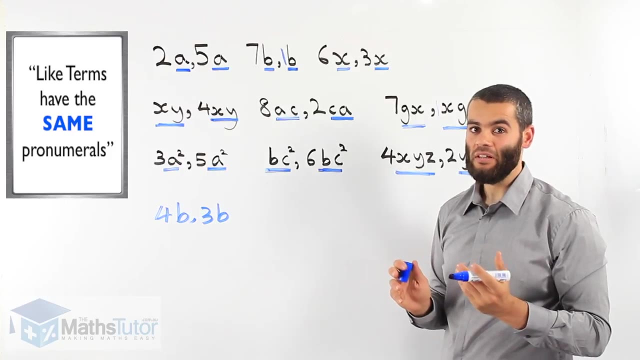 want to test you. I'm going to put some here and see which are like terms, which are different terms. Yes, I clearly could see which terms are like terms In the answer. you can check out these two and see whether you can figure them out yourself. we have 4b and 3b, well, do they? 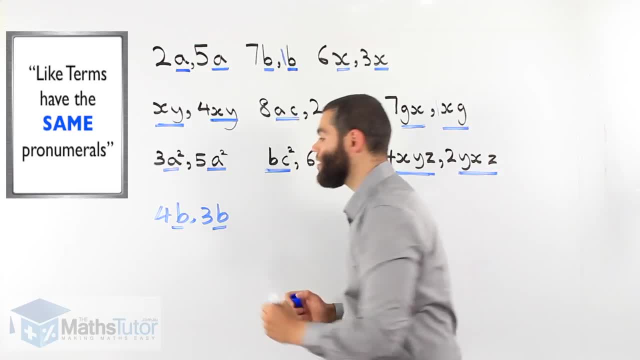 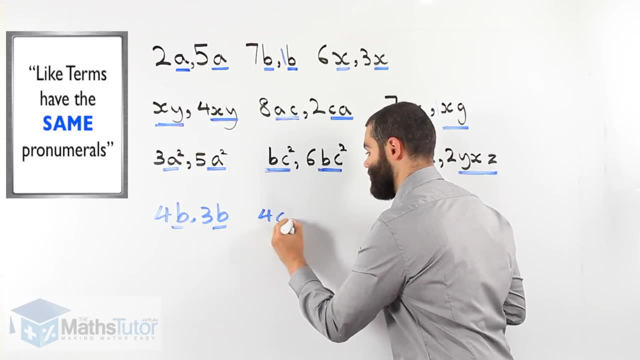 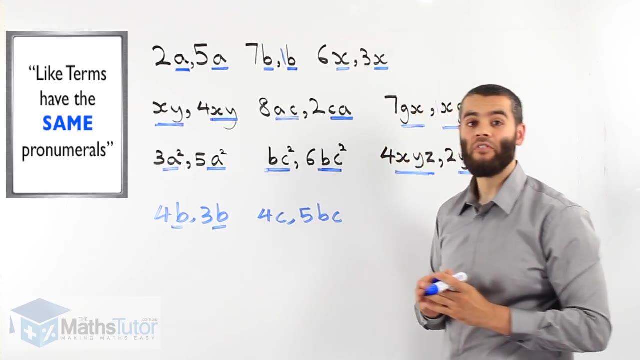 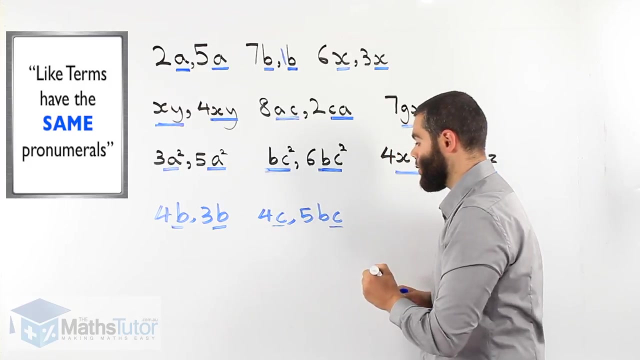 have the same pronumeral. yes, yes, then they are like terms. what about this one here, 4c and 5bc? well, are they like terms? we have a C here and we have a C here, but here we have a B and here we don't have a B. therefore, these are not like terms. 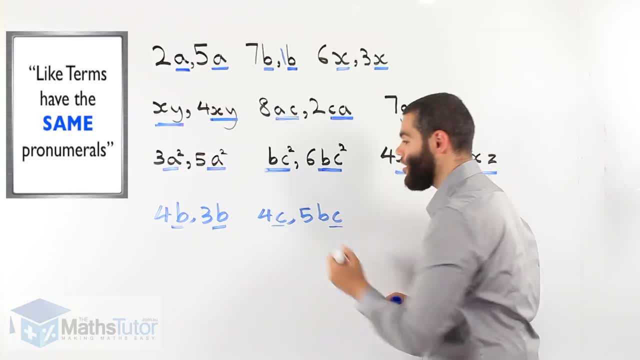 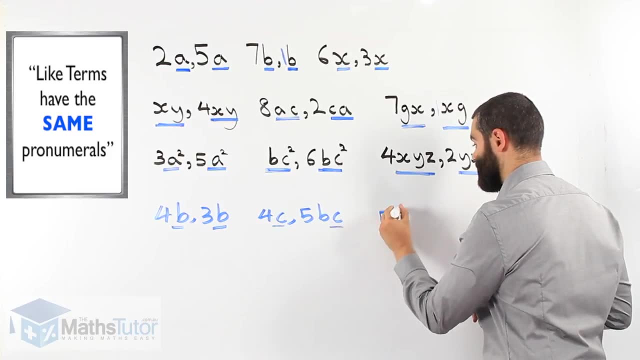 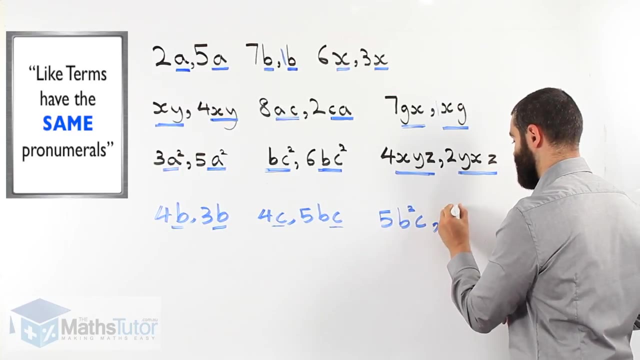 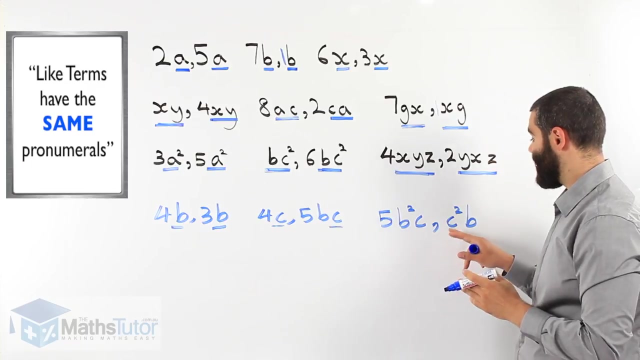 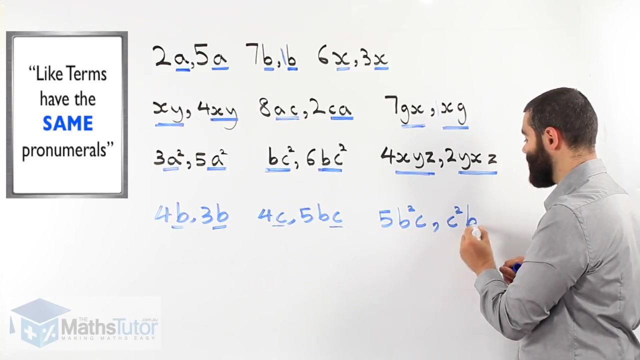 this is a term, this is another term, but they are not like terms because the pronumerals are different. what about this one here: 5b, 5b squared C and C squared B. so we have a term here, 5b squared C, and another term, C squared B. well, are they like terms we have? 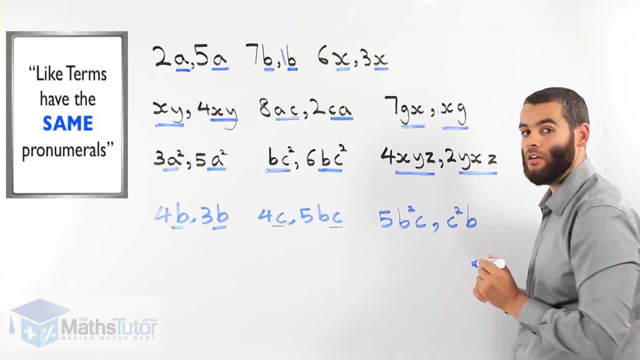 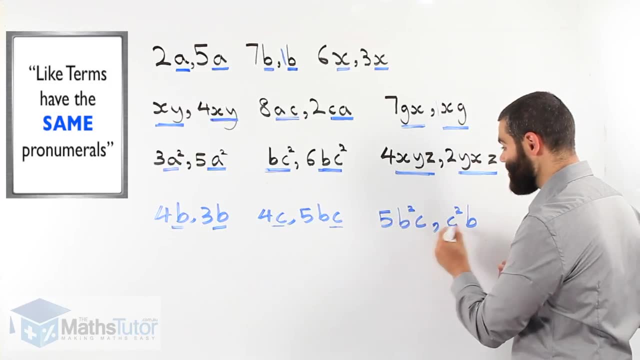 5b squared C and C squared B. well, are they like terms? we have a b squared and here we only have a b, while here we have a c and here we have a c squared. they are not like terms. why? because in reality 5 b squared is b, b, c. 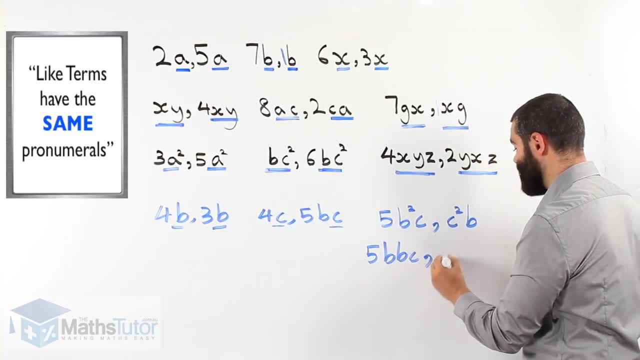 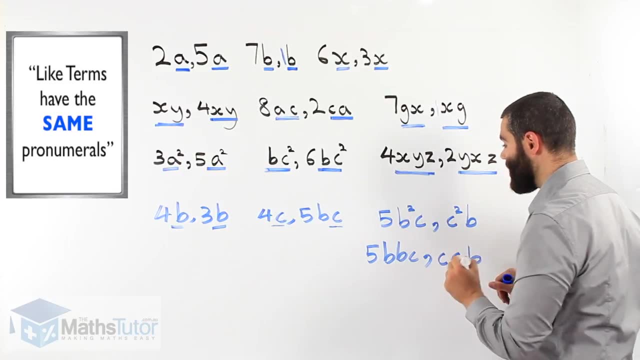 but we write it in simpler form and c squared b is really c, c, b, so they are actually different. they look the same, but don't get tricked with the squared. the squared here is on the b b times b, and the squared in this term is on the. 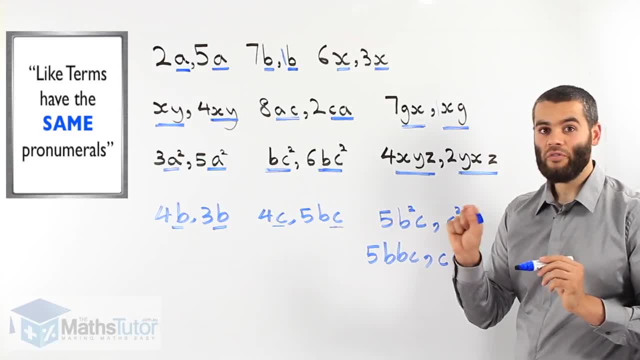 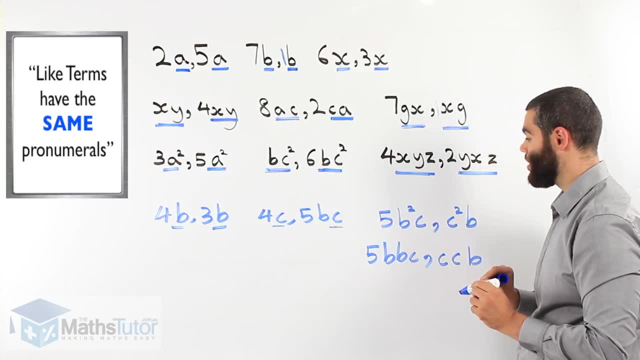 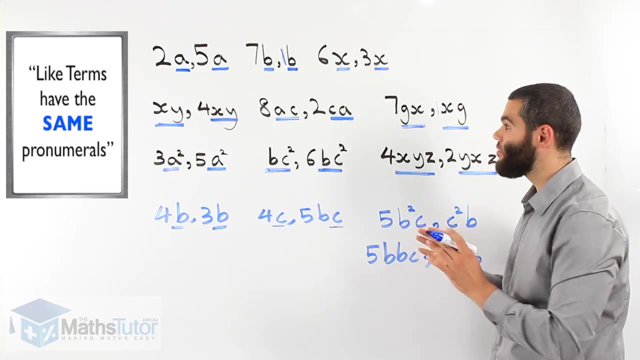 c c times c. so it's very important to differentiate. be careful, don't get tricked by. the squared has to be exactly on the same pronumeral. here it is actually different. so now we can tell what are like terms and we can differentiate between like terms and the terms that are not alike. now we can show. 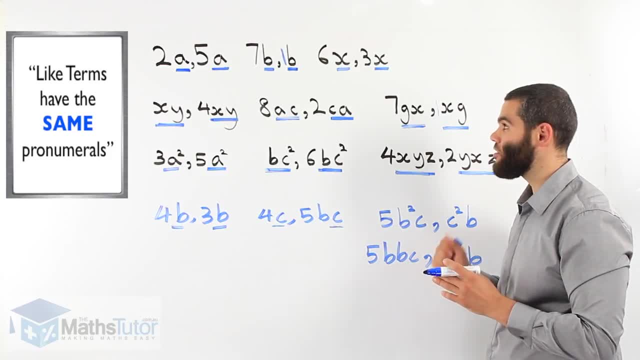 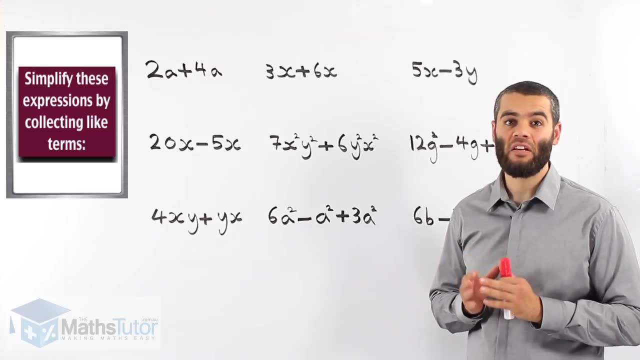 some examples of addition and subtraction of like terms in algebra. let's do that now. in these examples we are now asked to collect like terms. when we're asked to collect like terms actually means add and subtract the like terms only. remember the rule is: we can only add or subtract like terms. 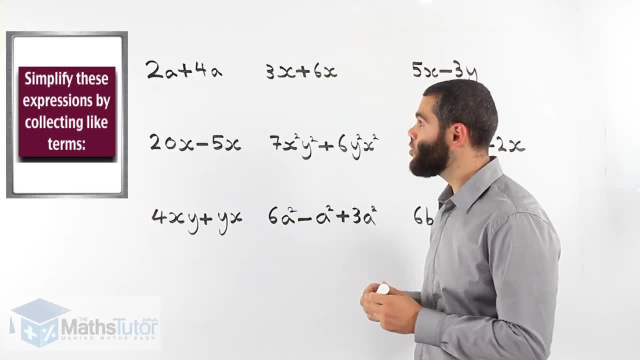 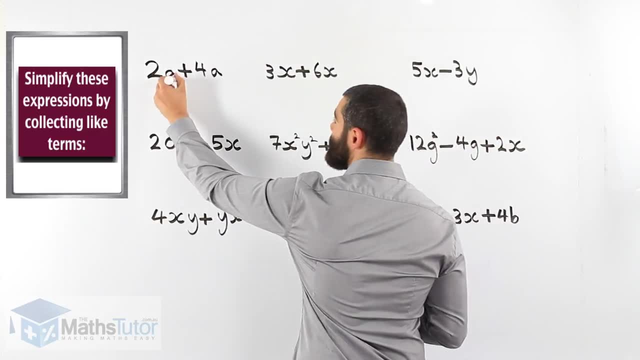 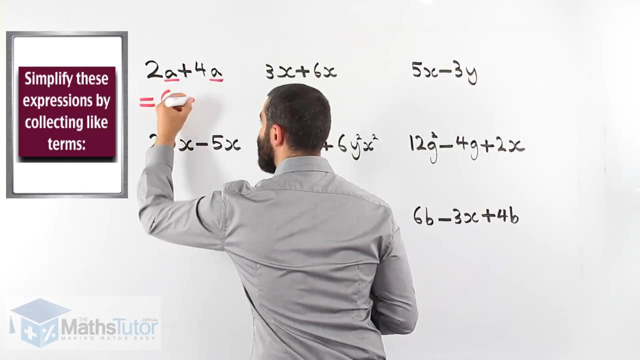 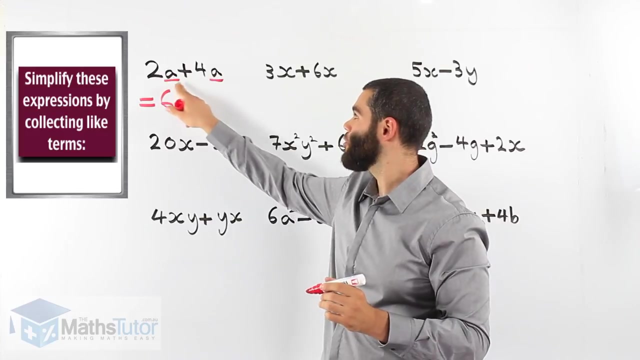 let's get started this example here: 2a plus 4a- are they like terms? well, do they have the same pronumerals? a and a? yes, 2a plus 4a, 6a- it's like saying two apples plus four apples- we have six apples- like terms, meaning they have the same pronumerals. 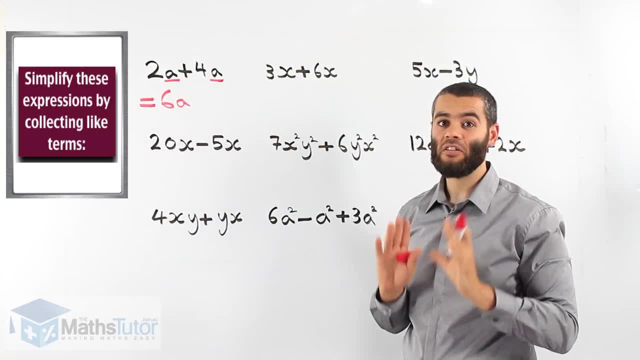 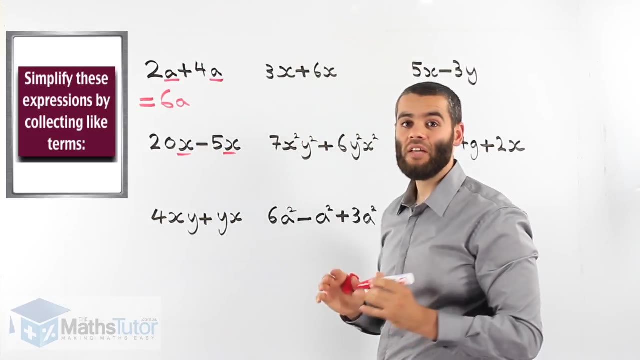 that means we can add them, because we can only add or subtract like terms. very, very important. rule: 20x, take away 5x. are they like terms? well, we have an x here and an x there. so, yes, they are like terms. so 20, take away 5. 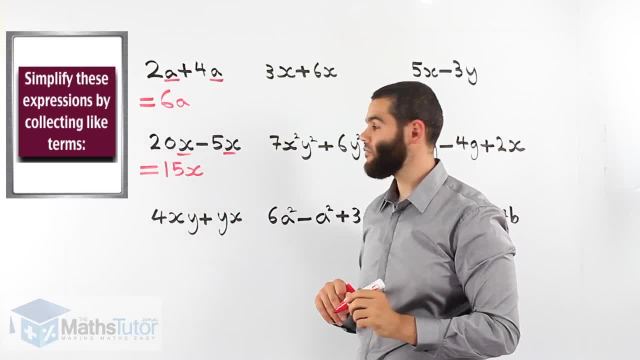 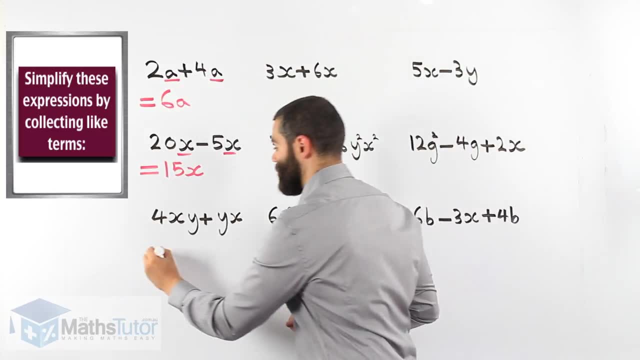 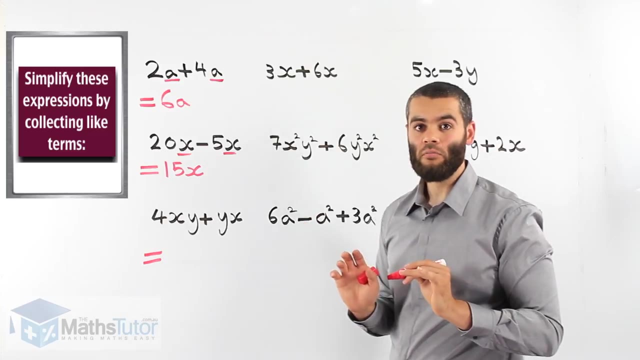 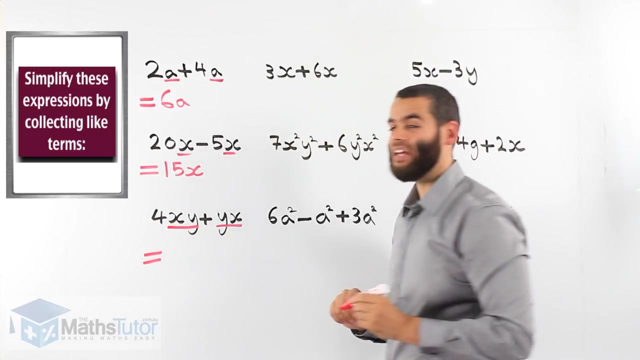 15x, 20x. take away 5x, 15x in this example. here we have 4xy plus yX. now are they like terms, because we can only add or subtract like terms: X, Y, Y, X. Yes, they are like terms. The order doesn't matter, as long as the. 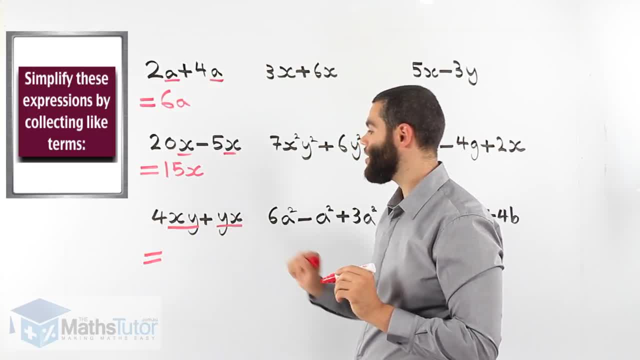 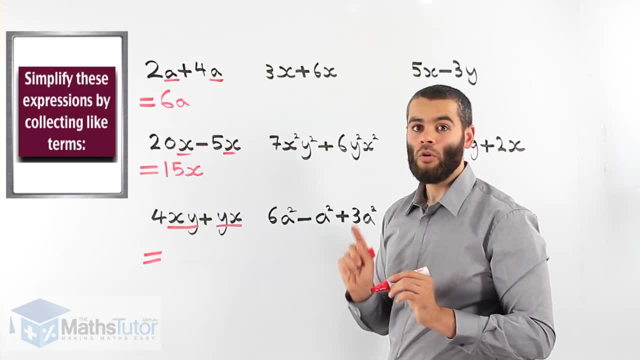 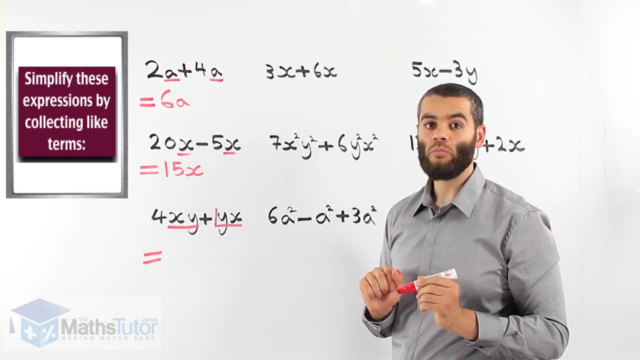 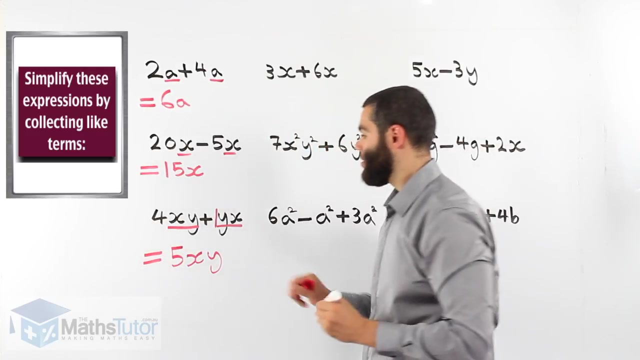 pronumerals are the same: X here, X, there, Y and Y. they are like terms. Now 4XY plus YX. We know that here there is an invisible one. Don't forget that. Make sure you remember there is an invisible one. 4 plus 1, 5XY, 4 plus 1, 5XY or 5YX. 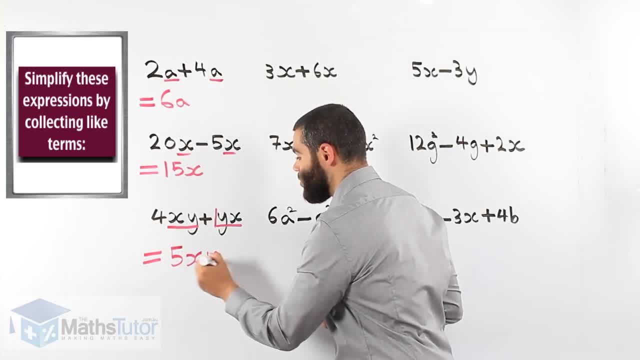 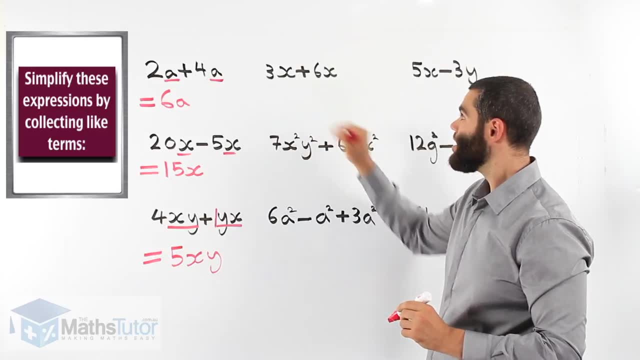 Doesn't matter. It's best to write it in alphabetical order: XY. so 5XY. 4 plus 1 is 5XY. Here we have 3X plus 6X. Are they like terms? Yes, they are like terms. They are like terms. Here we have 3X plus 6X. Are they like terms? 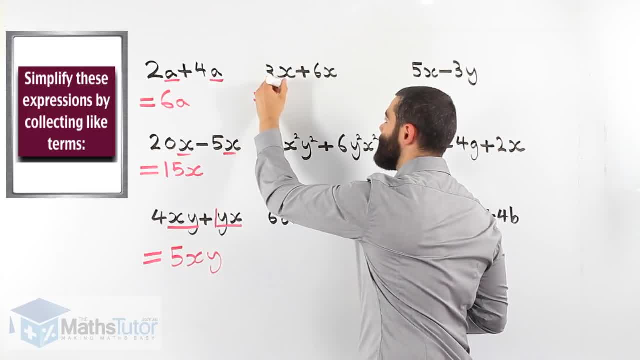 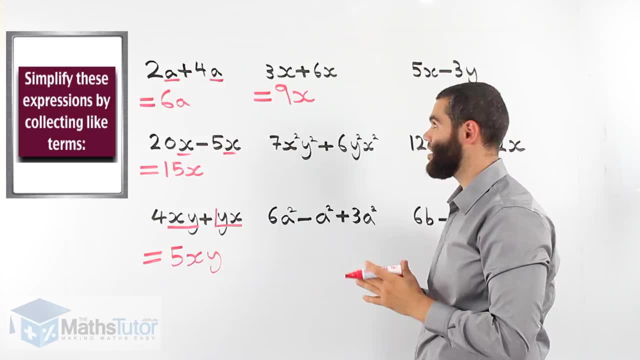 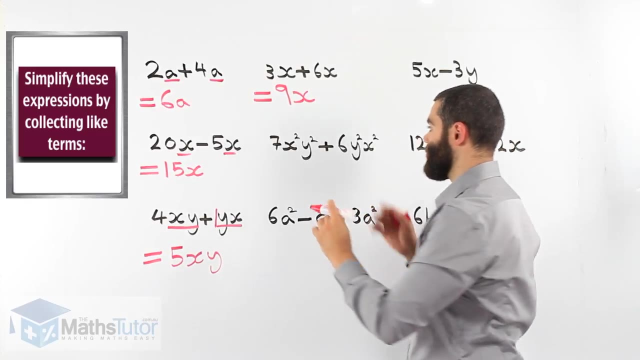 Yes, they are 3 plus 6, 9X, 3X plus 6X, 9X. It's like saying we have 3Xs on one side and 6Xs on another side. All together, we have 9Xs Here, 7X squared Y. 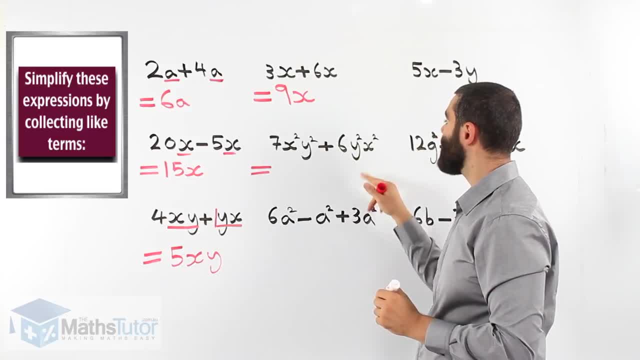 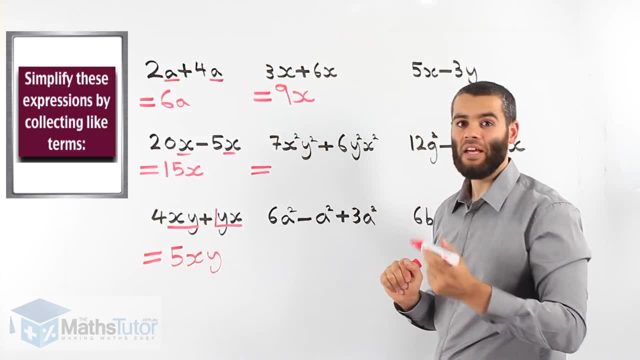 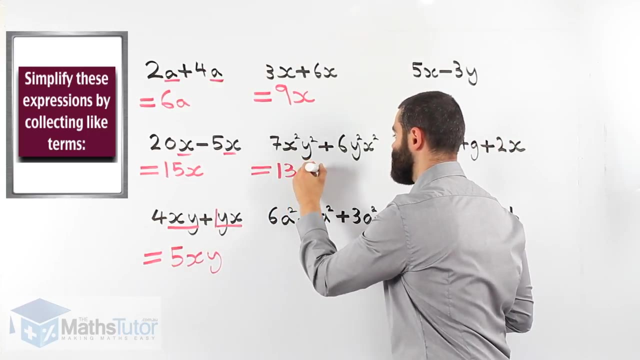 squared plus 6Y squared- X squared. Are they like terms? We have an X squared and X squared- Yes, Y squared and a Y squared- Yes, That means we can add the 7 and the 6.. We have 13X squared- Y squared. Now we have 3. 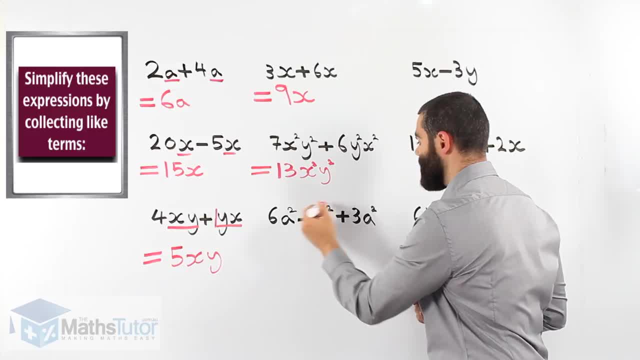 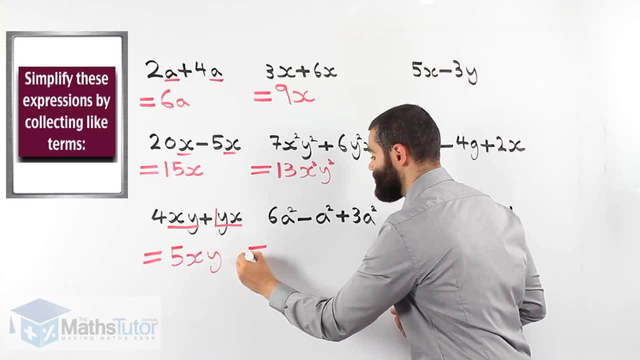 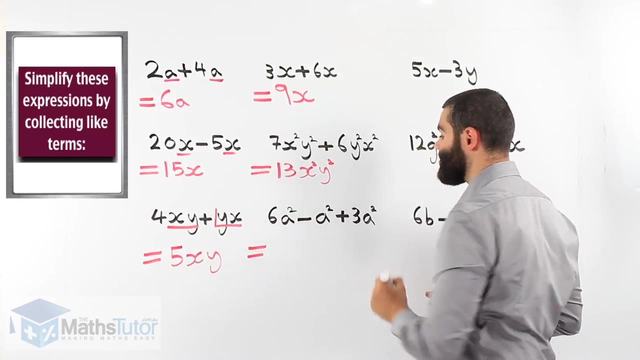 terms. We have a term here, another term there and another term there, And we, what we are asked now to collect them so we can add or subtract them. Do they have like terms? Let's see A squared, A squared, A squared. Yes, they are all like. 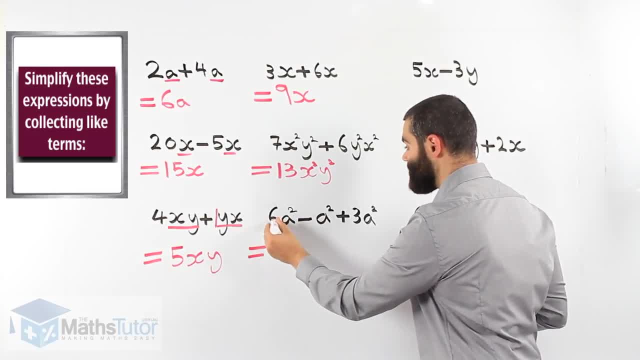 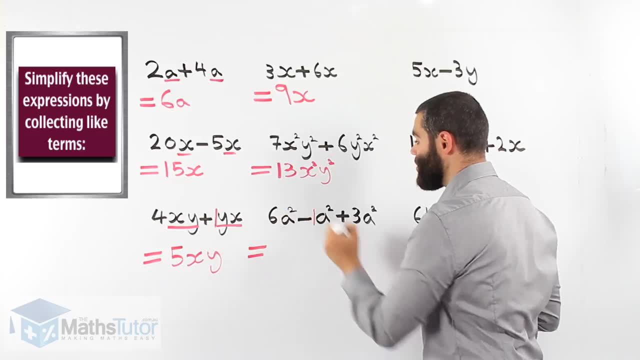 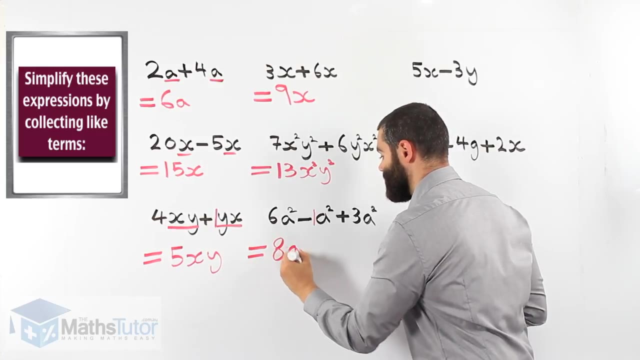 terms. We can now collect them. 6 take away. Now we said, in front of the A squared there is an invisible 1.. 6 take away: 1 is 5.. 5 plus 3 is 8A squared. So 6A squared minus 1A squared. 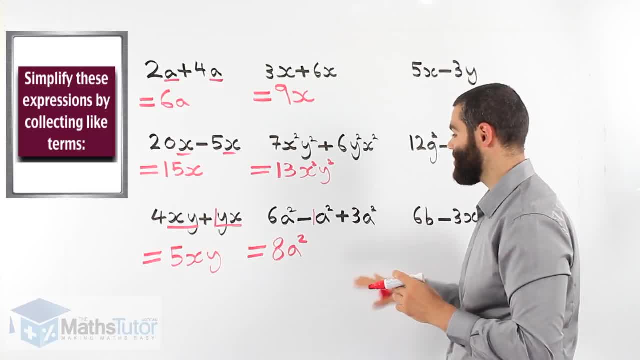 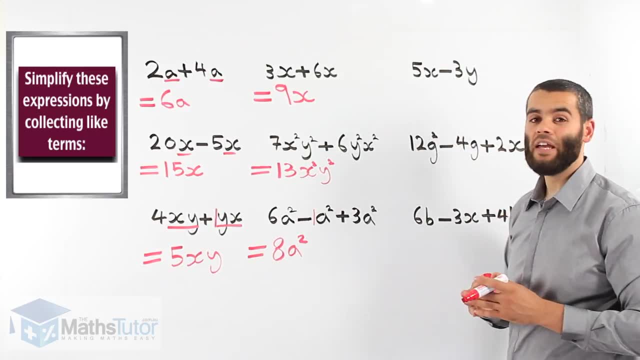 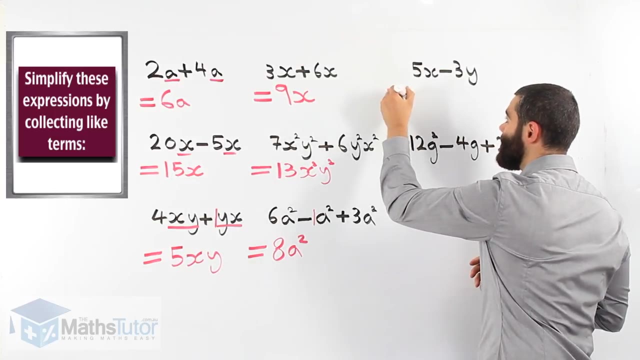 is 5A squared. 5A squared plus 3A squared is 8A squared. This question: 5X take away 3Y. they are asking us to collect like terms. Well, let's see: 5X take away 3Y, Hang on. 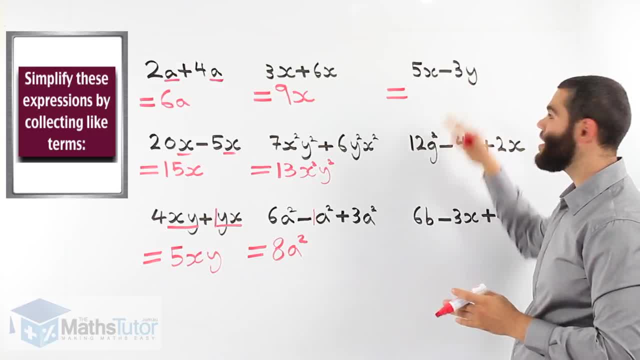 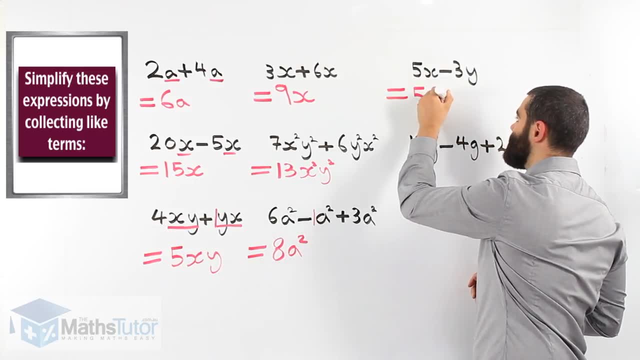 these aren't like terms. We have an X here, we have a Y here. they are different, They're not like terms, So we can't actually collect them. So guess what? The answer is the same as the question. Nothing changes. 5x. take away 3y. That's as simplified. 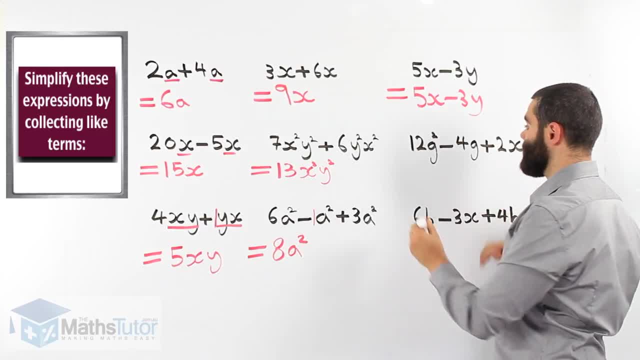 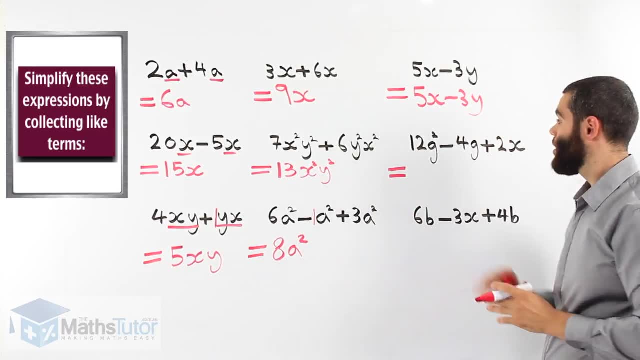 as it gets This here. you need to make sure you switched your brains on and you are concentrating: 12g squared minus 4g plus 2x. Well, any like terms? We look and we notice there is no like terms. This has a g squared, this term has g squared, this term has g and this term has.